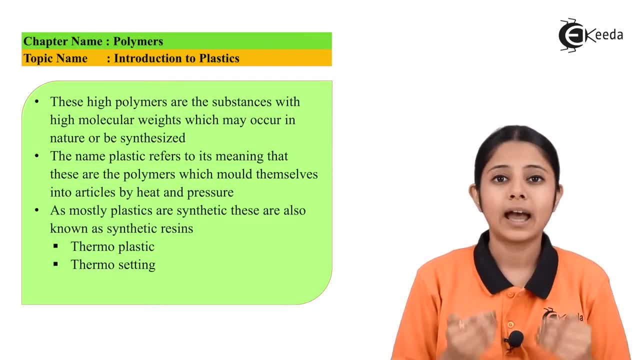 Macro means smaller and macro means larger. So when I am talking about a macromolecule, I mean a large molecule, a molecule with high molecular weight. It has many small molecules and atoms combined together and these dense molecules come together and form a macromolecule. 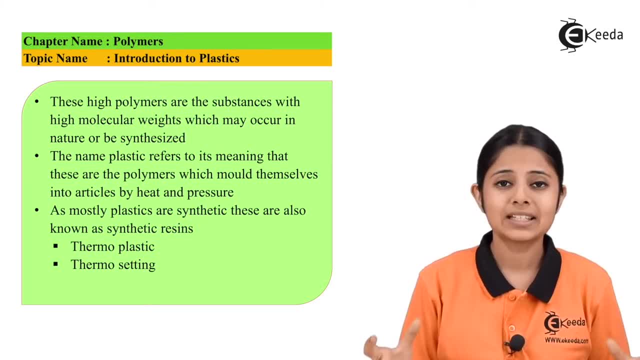 These macromolecules are known as monomers. Many such monomers combine together and form a polymer, and this polymer is nothing but plastics. Plastics can be both natural as well as synthetic. Generally, we use synthesized plastics on a daily base, and these plastics have replaced metals in 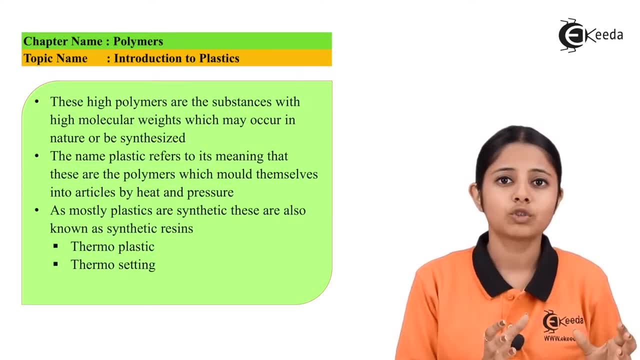 various purposes. For example, before people used to use metal boxes for lunch boxes. They were made up of steel, they were made up of copper, they were made up of aluminium, But now people use plastic boxes. And there are many such examples wherein plastics have replaced many other elements. 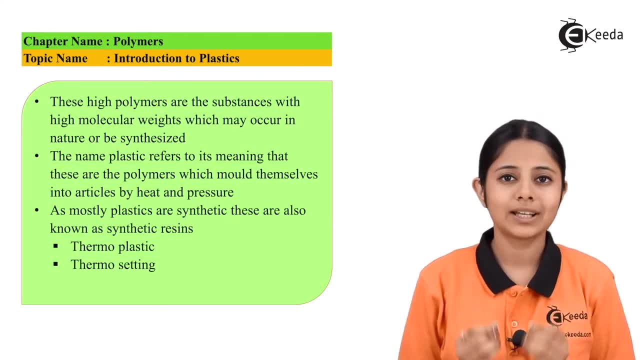 and substances for our daily, day-to-day use. So now, what exactly are plastics? Plastic is a substance which can mold itself into any article if proper amount of heat and proper amount of pressure is given. So these plastics are synthetic plastics. What do we mean by synthetic plastics? 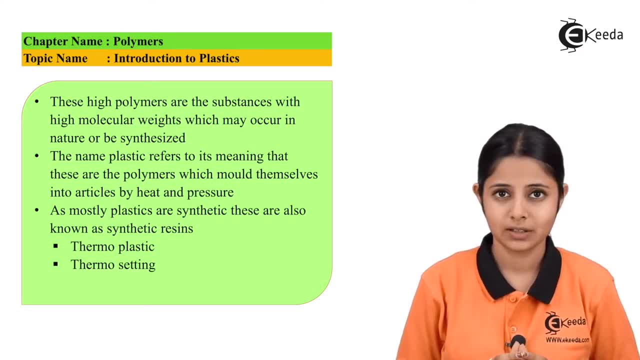 Plastics which are made by human beings. They are man-made plastics, And these man-made plastics can mold themselves by heat or pressure into any kind of material we want or any kind of articles we want. These synthetic plastics have a name and they are known as synthetic resins. These 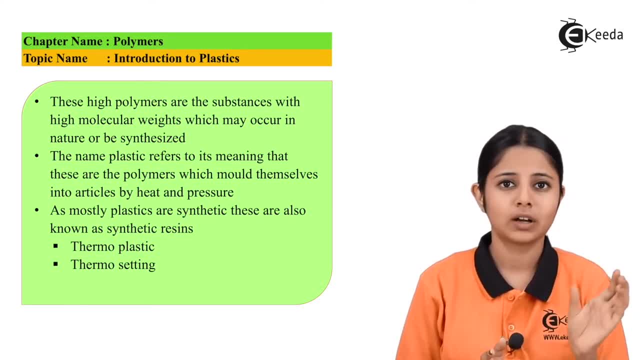 synthetic resins can be subdivided into two types. One is called a synthetic resins and the other one is called a thermosetting resins. These are made up of plastic, which are made up of two parts: Thermoplastic plastics and thermosetting plastics. Thermoplastic plastics also have a different name. 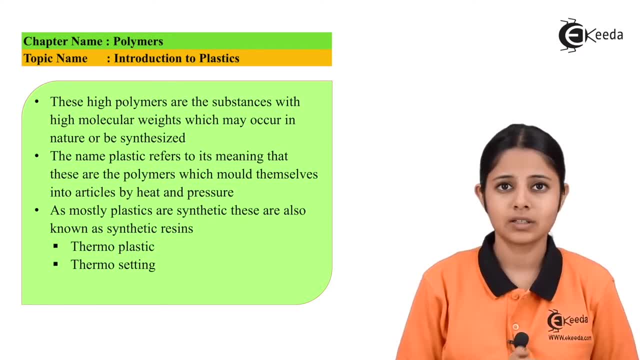 known as thermosoftening plastics. These are the plastics which we take the material and we heat the material. It will soften, it will get liquidified and we can pour that liquid into a mold or any article and we get the article or the product out of it. If we do not like the shape of 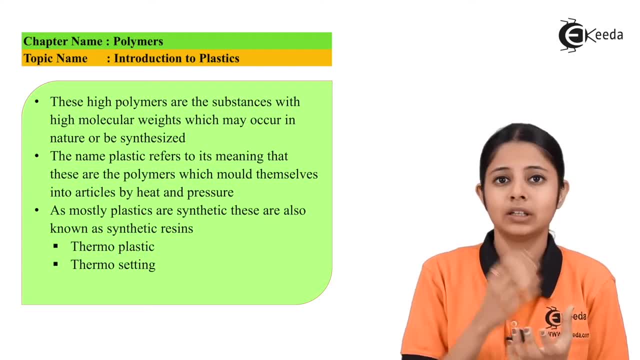 the product. we can again reheat the entire product. The product will again become a liquid, and then we can pour it again into another mold. That means, on heating it will just become liquid, On cooling it will harden. For thermosetting plastics we can do it just once for the first.